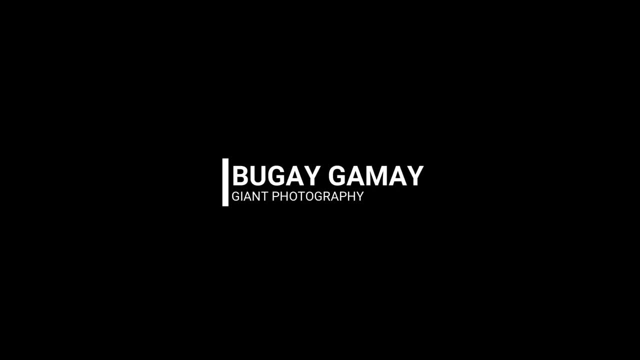 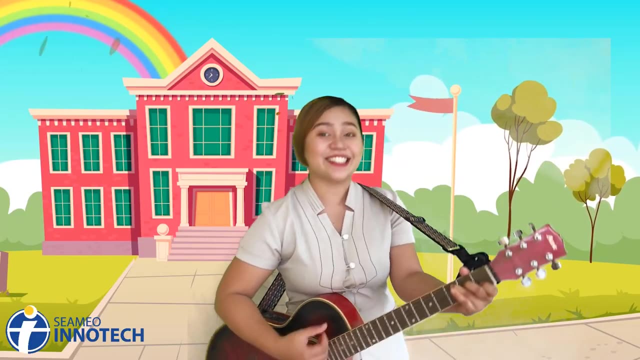 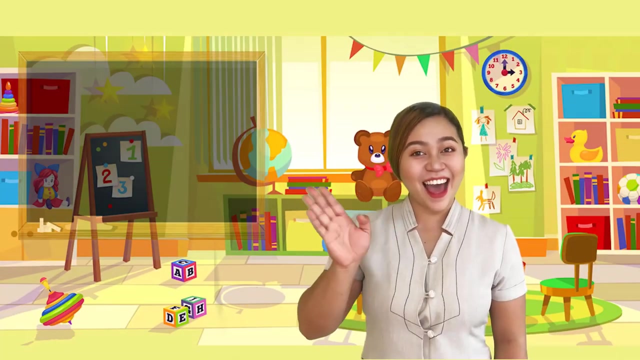 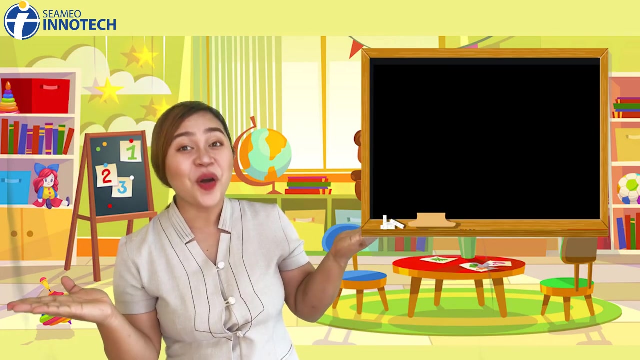 Hello, hello, hello, hello. how are you? It's nice to be with you and you and you and you. Hi, I'm Teacher Psyche. Welcome to our class. Today we will learn about the four kinds of weather. 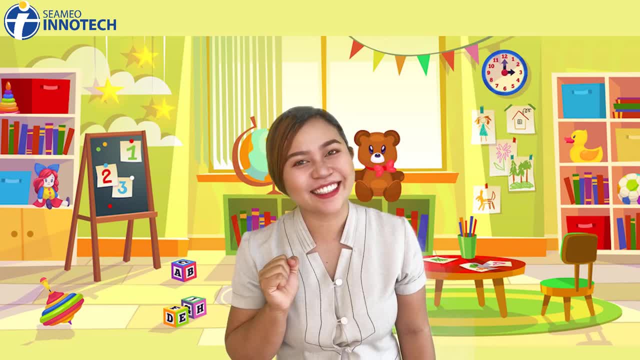 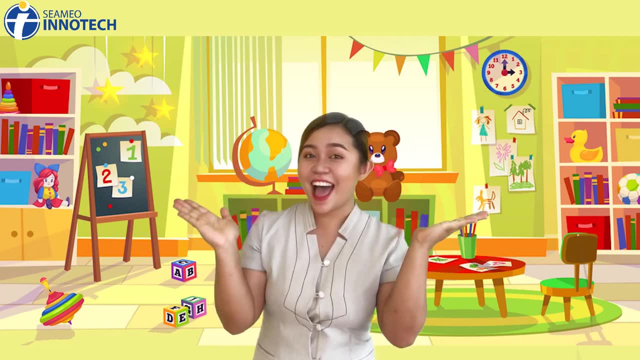 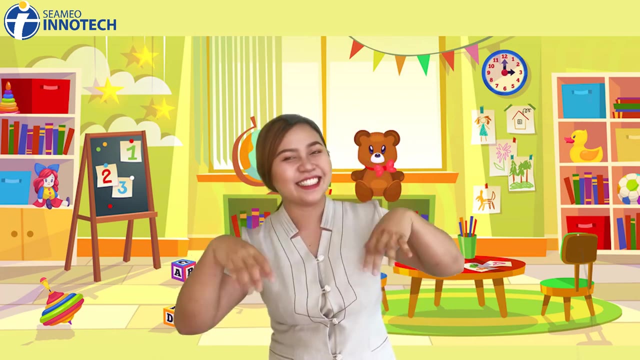 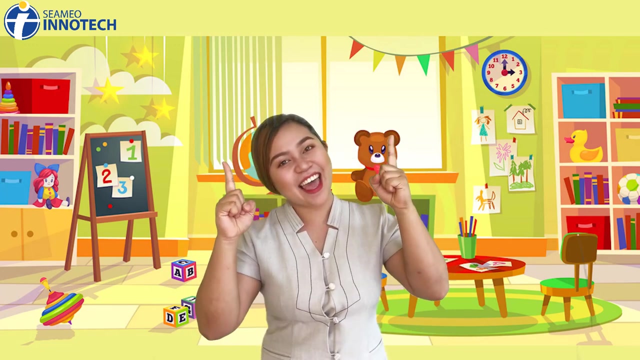 First, let's sing a song: How's the weather? How's the weather, How's the weather today? Is it sunny, Is it rainy, Is it cloudy, Is it windy? How's the weather today? Yay, Great singing. 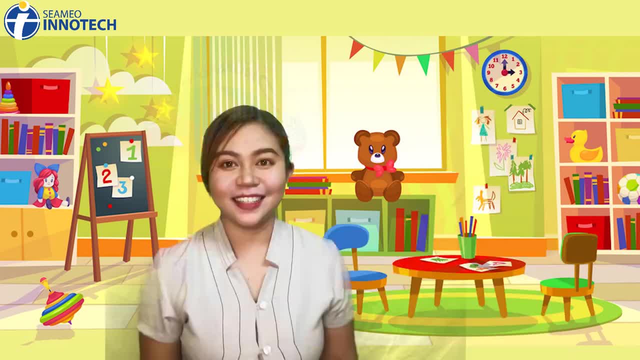 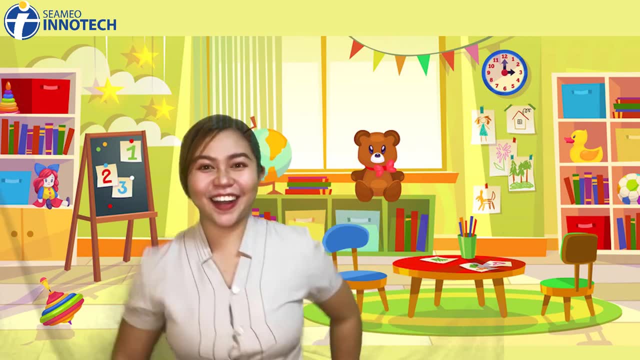 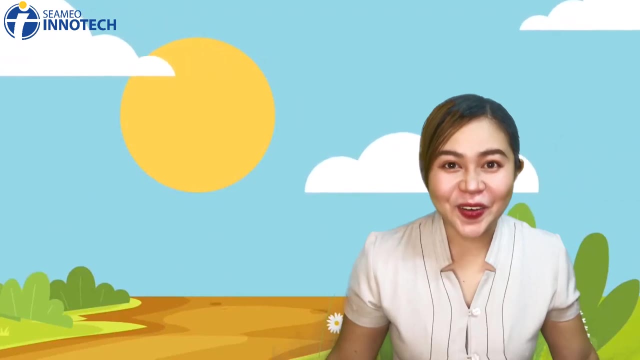 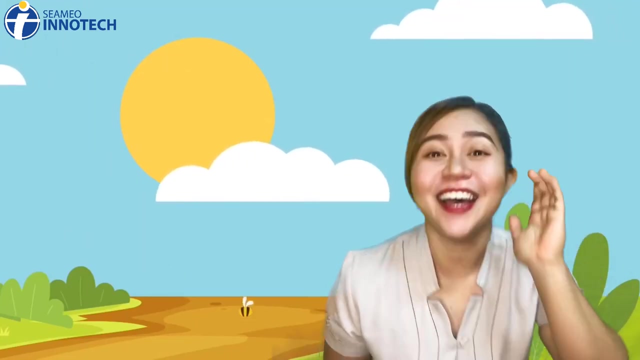 Here's your singing song. We have four kinds of weather. Let's learn more about them. Let's go. Wow, I see something round and yellow. What is it? You're right, It's the sun. Yay, Yay. Here's your song. 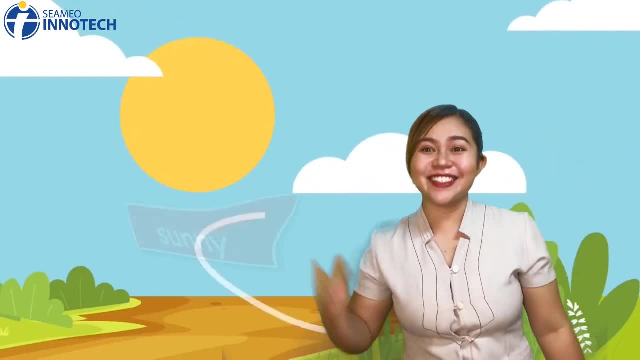 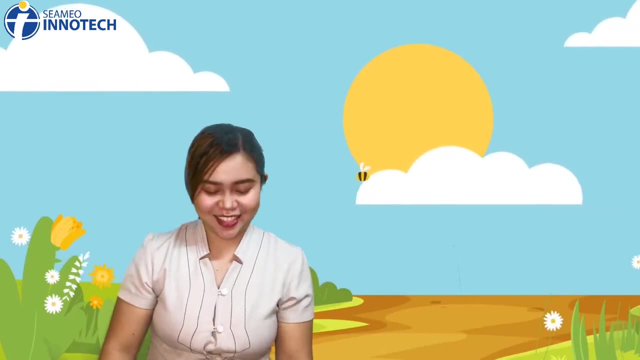 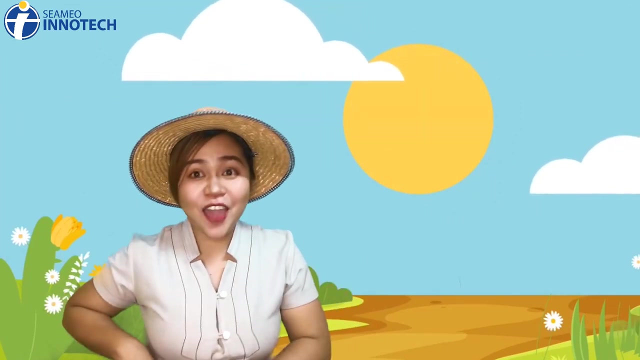 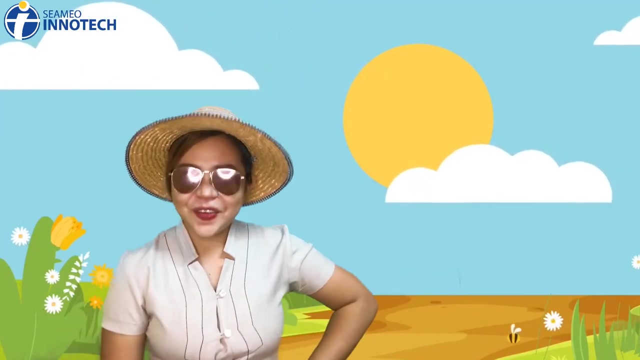 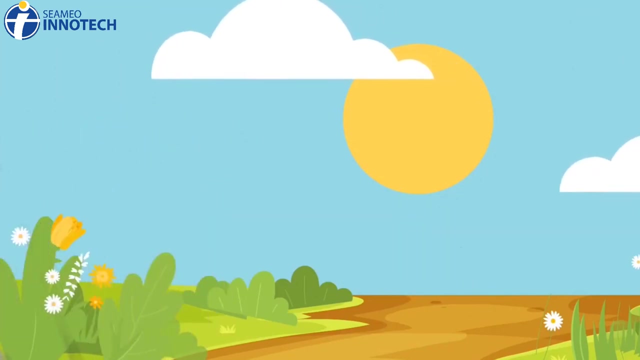 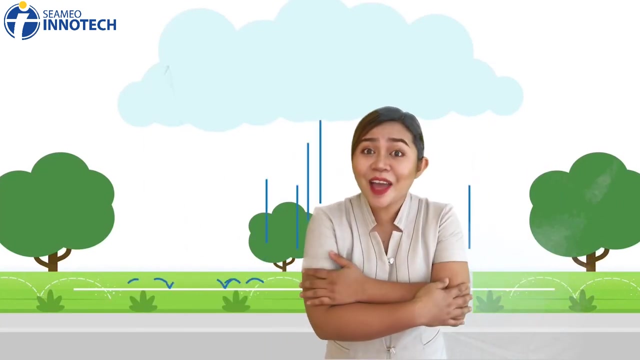 The weather is sunny because the sun is shining brightly. I have a hat. It's perfect for a sunny weather. I almost forgot I have sunglasses here. Wow, This is nice for a sunny weather. Let's go. Oh no, It's raining And I'm getting cold. 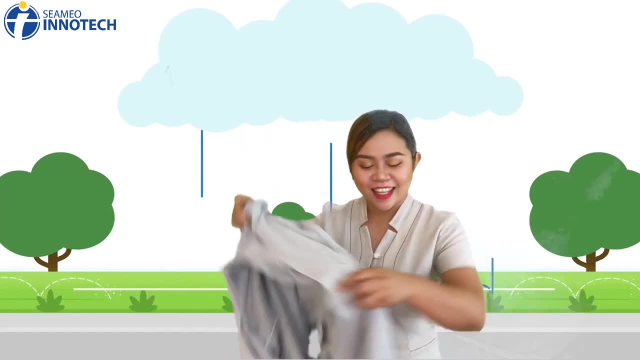 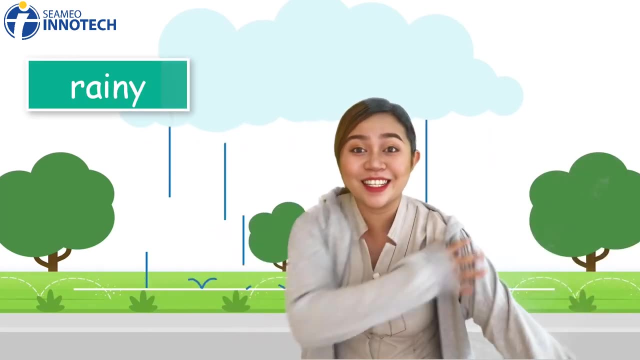 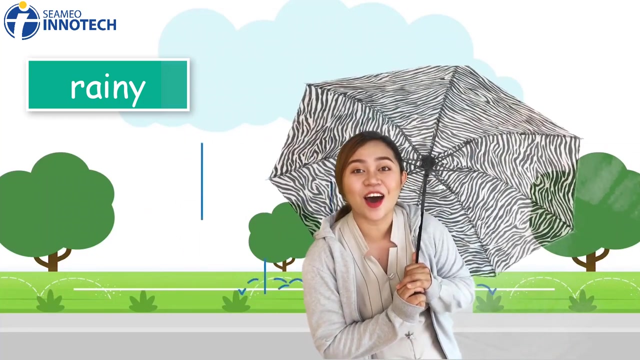 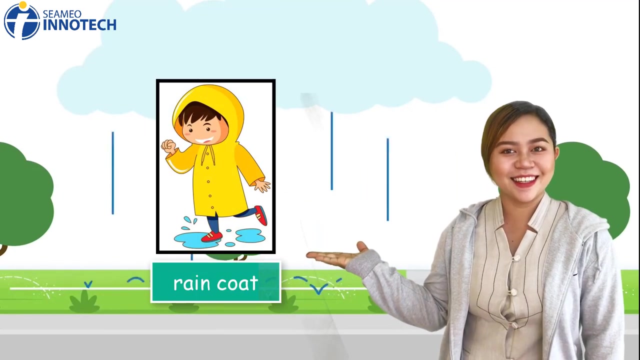 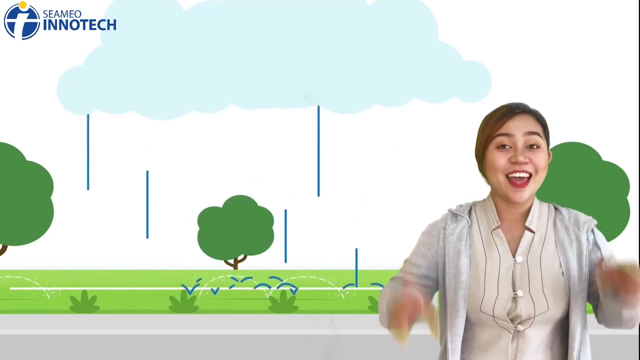 Good thing I have a jacket. It will keep me warm in this rainy weather. Also, it is important to use an umbrella, just like mine. It will keep you dry on a rainy weather. You can also wear a raincoat or boots. It will help you stay warm and dry in this rainy weather. 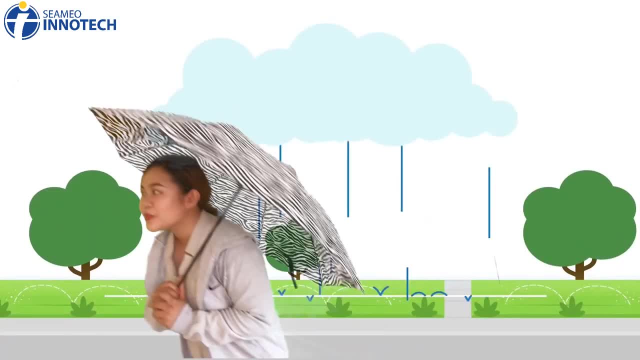 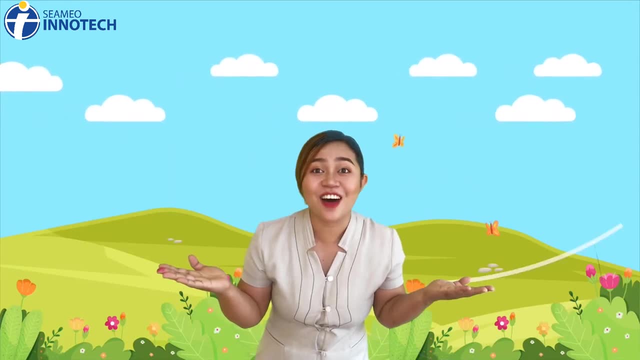 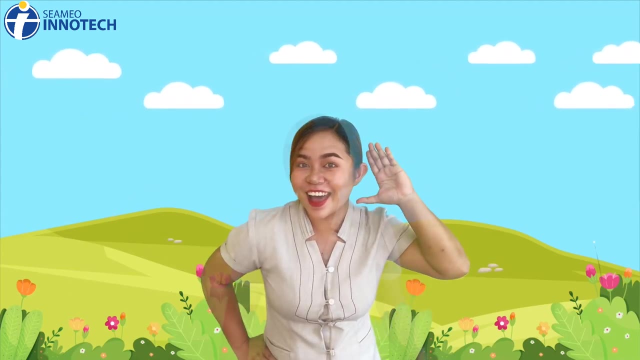 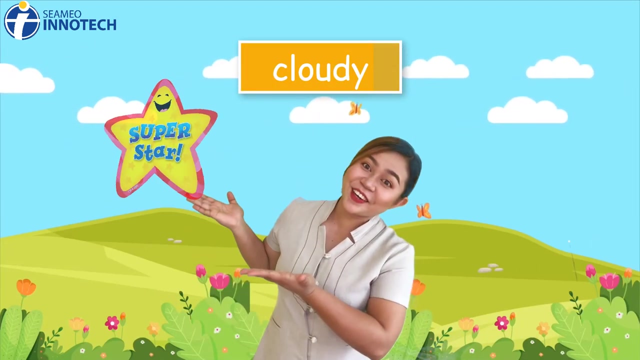 Let's go. Wow, There are many clouds in the sky. What weather is this? Wow, There are many clouds in the sky. What weather is this? What weather is this? It's very good. It's cloudy. Another star for you. 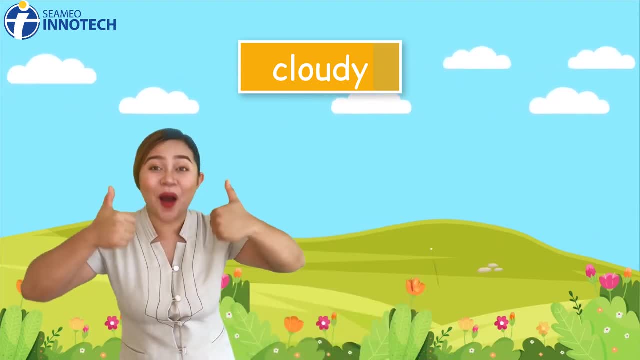 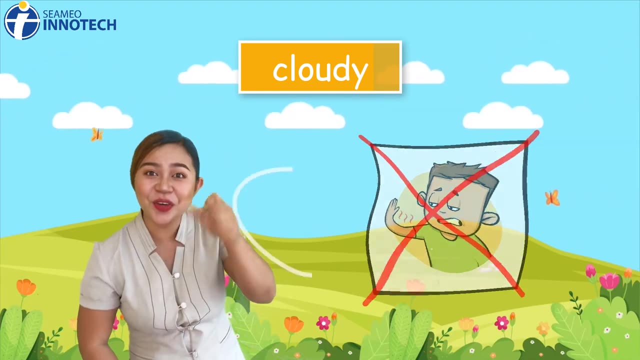 Another star for you. A cloudy weather like this is perfect for playing outside. It will not cause sunburn. It will not cause sunburn And you won't need a hat because it's not warm and sunny outside. And you won't need a hat because it's not warm and sunny outside. 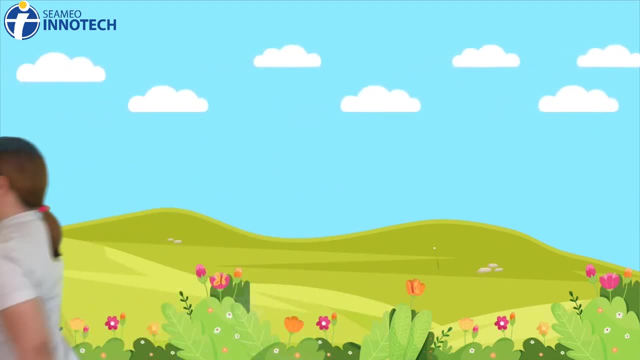 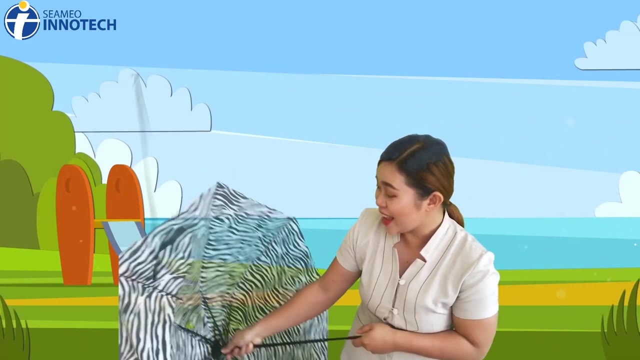 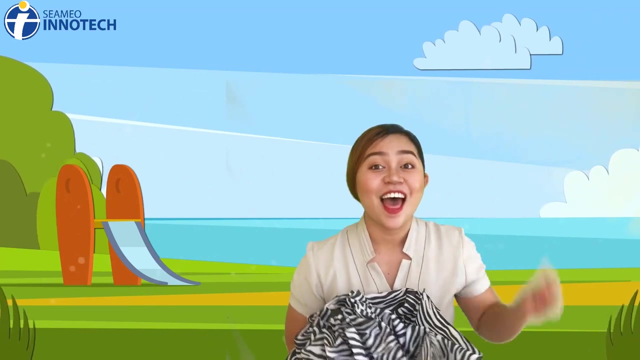 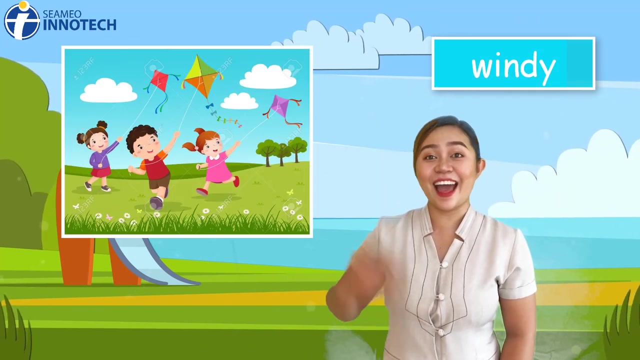 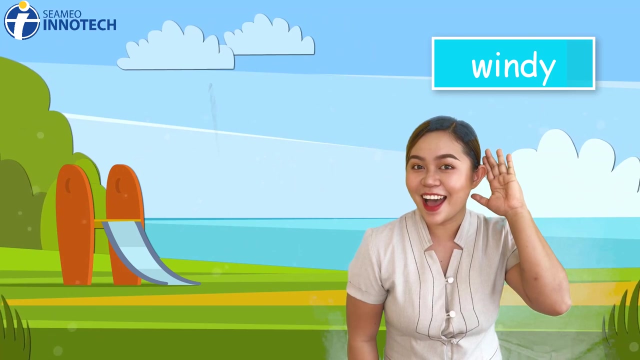 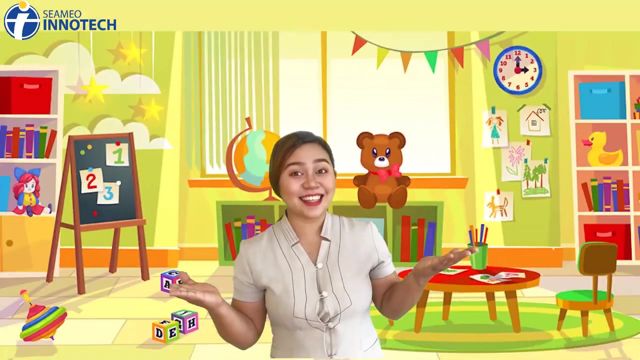 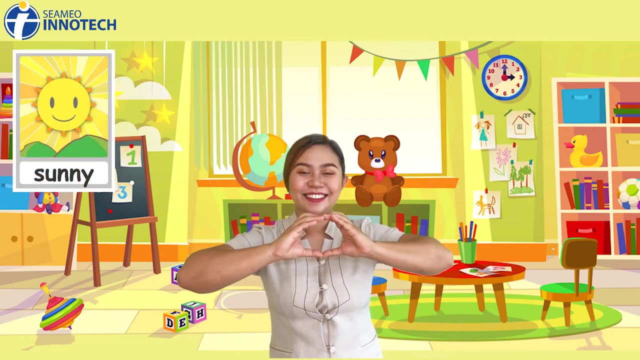 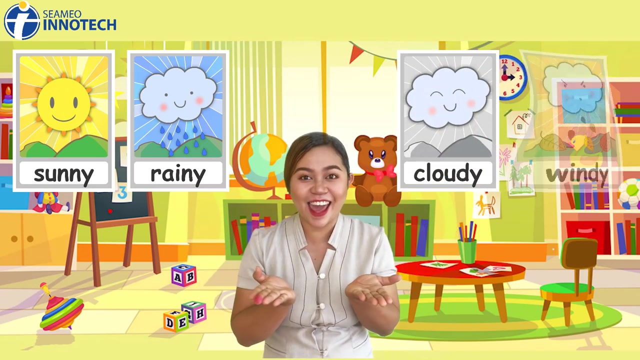 Let's go go. the wind is blowing very strong. that means this is a windy weather. it is nice to fly kites on a windy weather. do you like to fly kites? wow, that's great. I like flying kites too. let's say the four kinds of weather again: sunny, rainy, cloudy and windy. 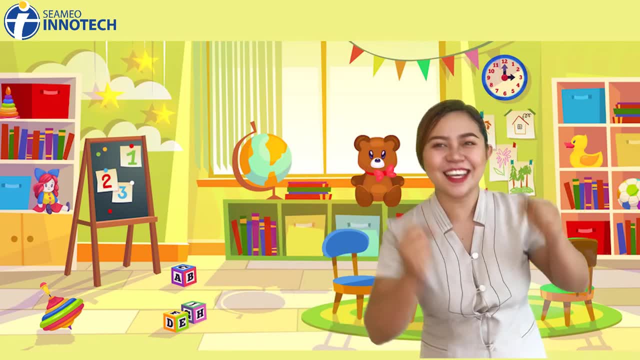 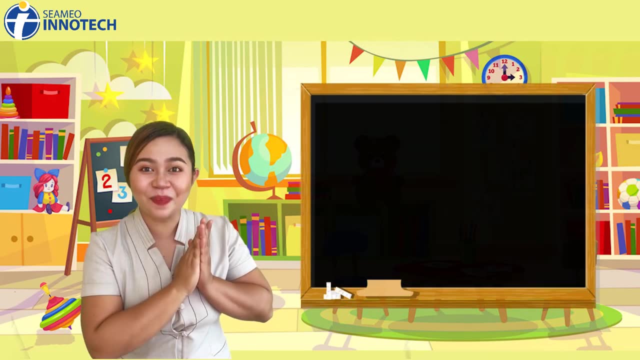 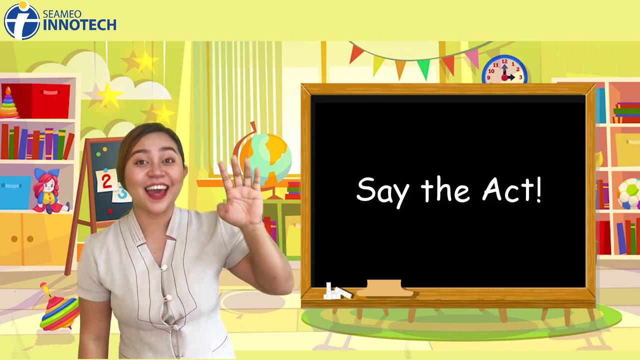 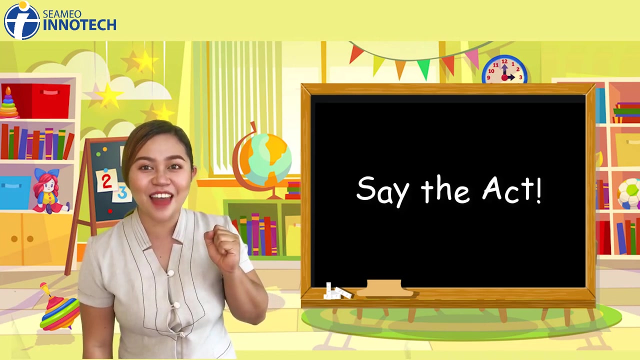 hooray, you did a great job. here's your weather sign. let's play a game. teacher Psyche will show you pictures of the four kinds of weather and I will also do some actions. you will tell me the name of that weather. are you ready? great? 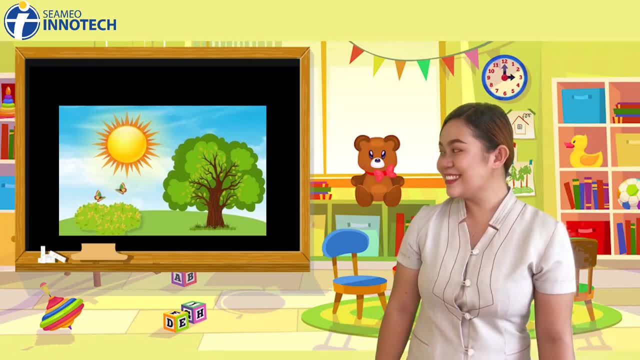 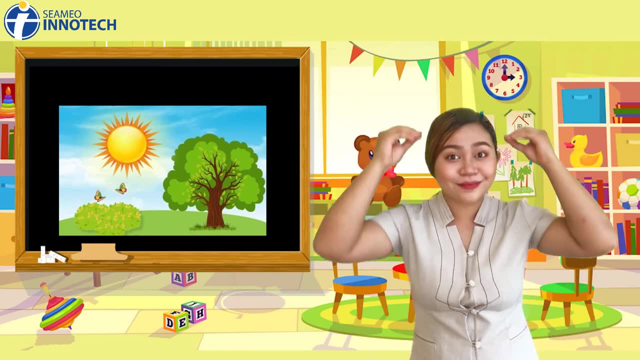 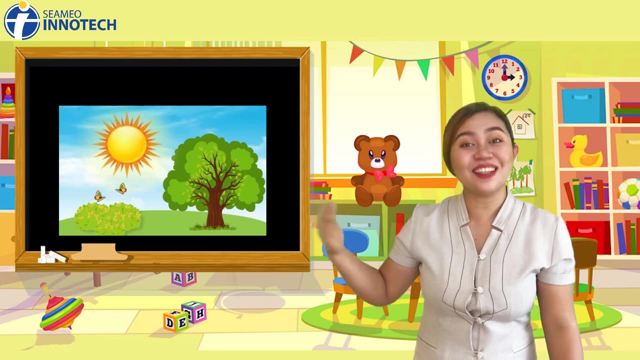 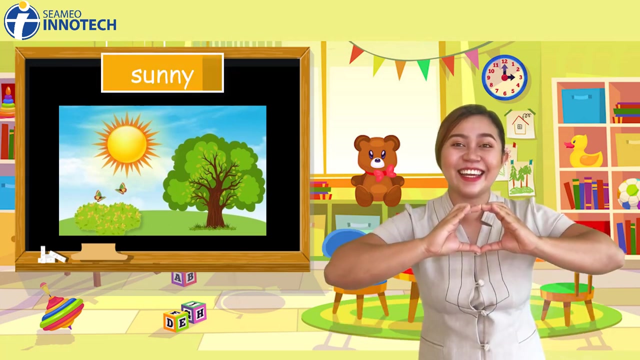 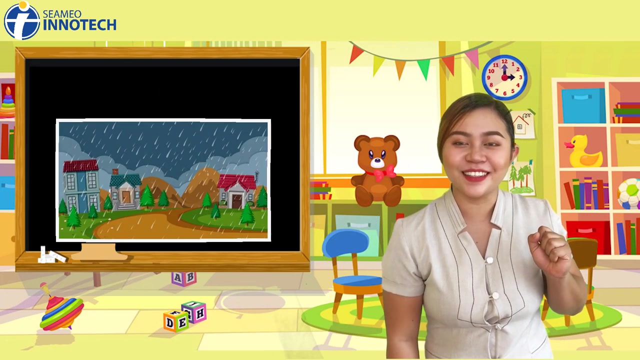 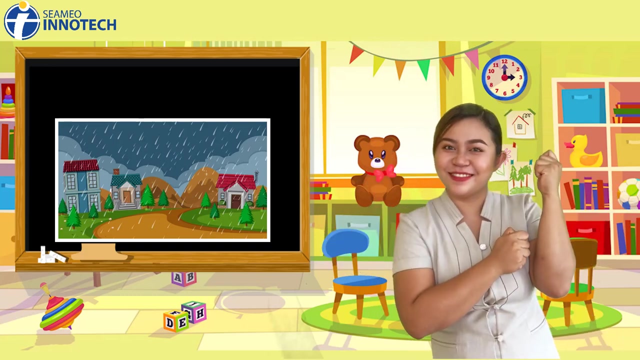 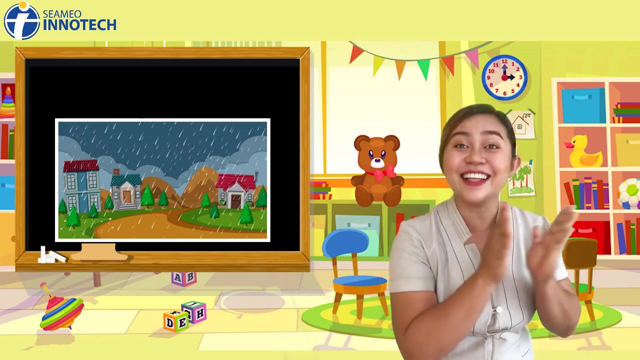 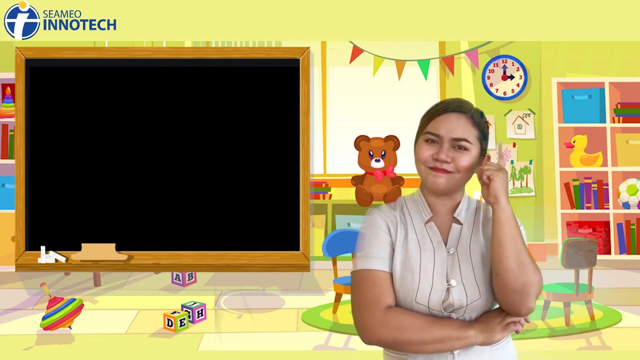 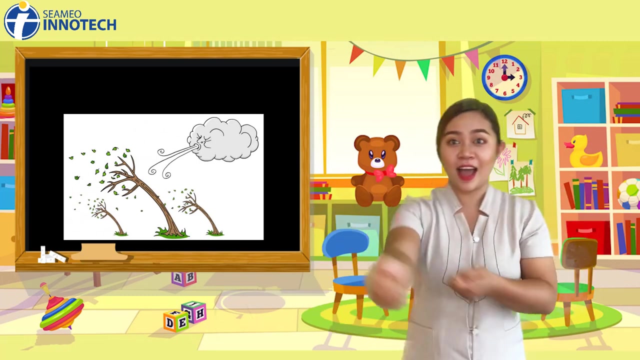 great, Let's go. What weather is this Amazing Sunny. Here's your star. Yay, Now try this one. What weather is this? Well done, Rainy. Here's your rainy star. What is this? Well done, Rainy. Here's your windy star. 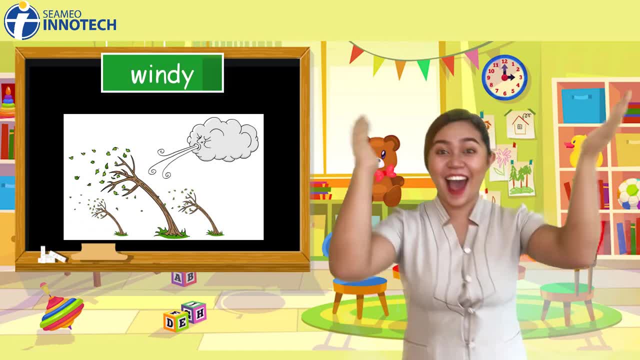 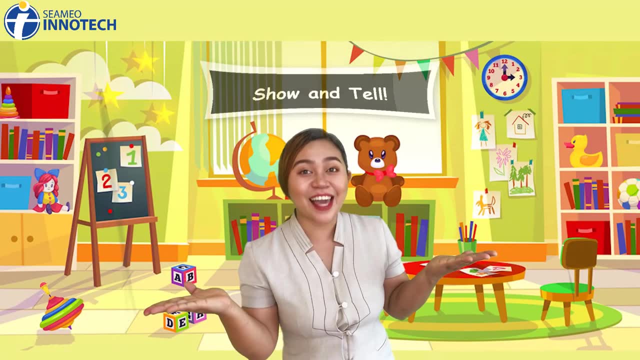 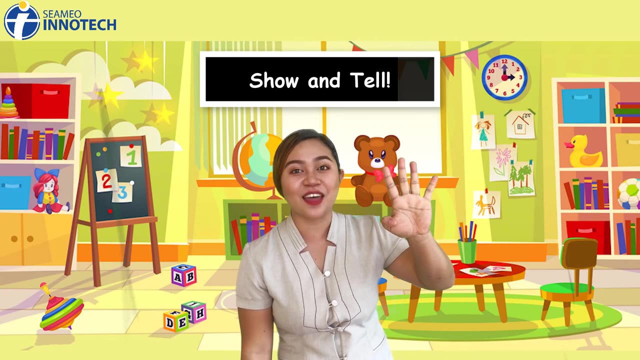 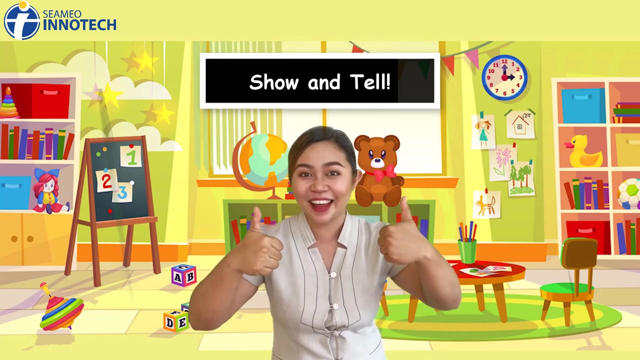 Excellent, It's windy. Yay, Here's your windy star. Now let's play. show and tell. Teacher will show you again pictures of the four kinds of weather and you tell me what can we do for that weather. Are you ready to play? 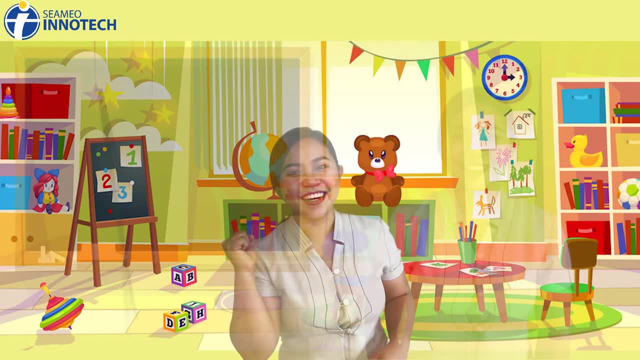 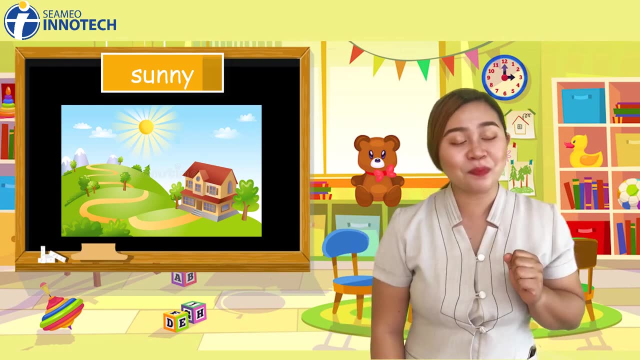 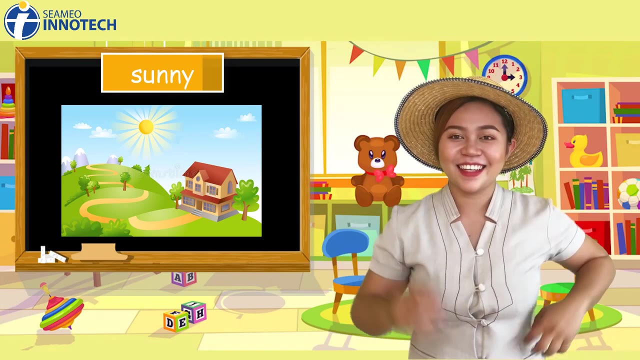 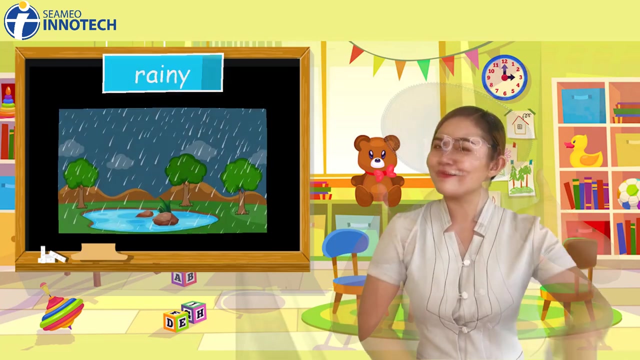 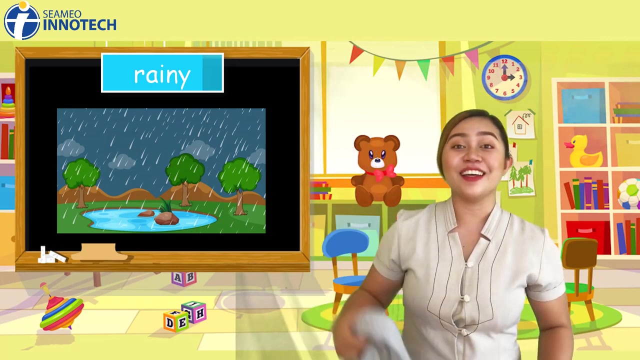 Amazing, Let's go. That's right. We can go to the beach or the pool on a sunny weather, And we can wear our hats And sunglasses too. Well done. We can use a jacket or an umbrella to keep us warm and dry on a rainy weather. 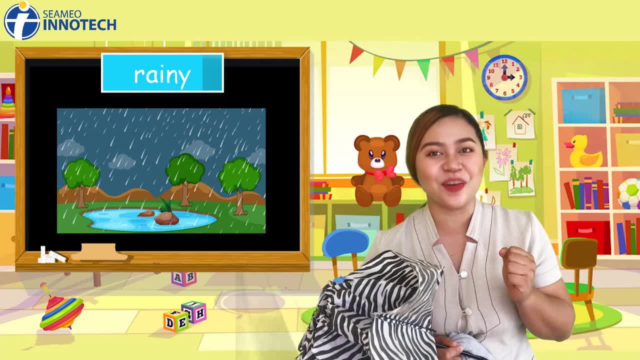 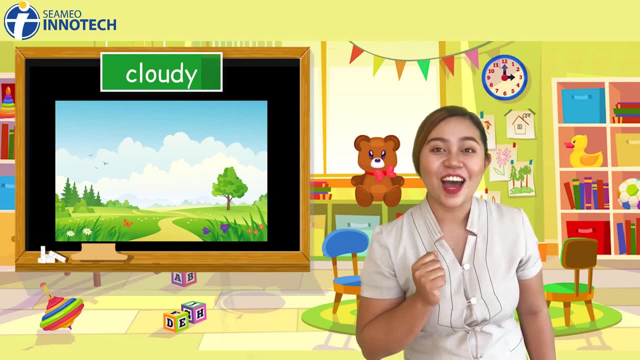 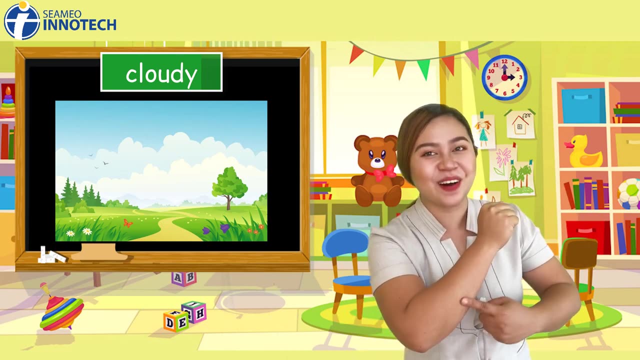 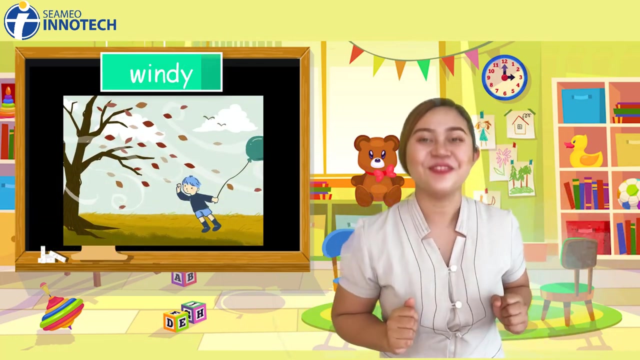 And yes, we can wear a raincoat and boots too. Way to go. Yes, On a cloudy weather, we can play outside without getting any sunburn. Yay, Amazing work. Last one Very nice. On a windy weather, we can fly our kites.